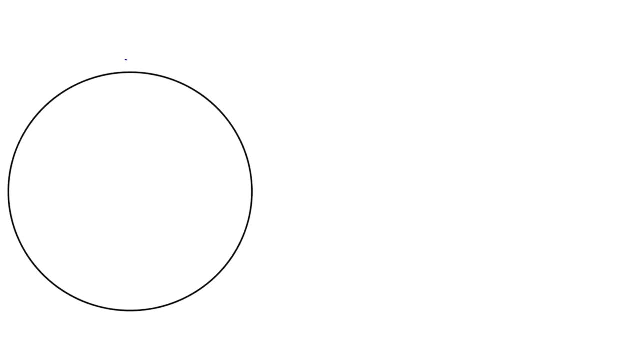 what this video is for. So let's draw a wheel here. If this wheel rotated one time, that would be one revolution, which is equal to 360 degrees of rotation, and that's also equal to 2 pi radians of rotation. So usually it's pretty quick to switch between these. but 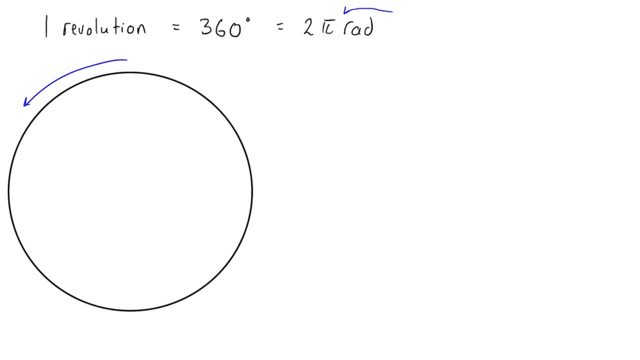 just to clarify any abstraction here: 2 pi it's just 2 times pi, that's equal to 6.28 approximately radians. So if you really don't like using the pi symbol, you can calculate it out and just truncate some decimal places. but anytime you're able to, you should. 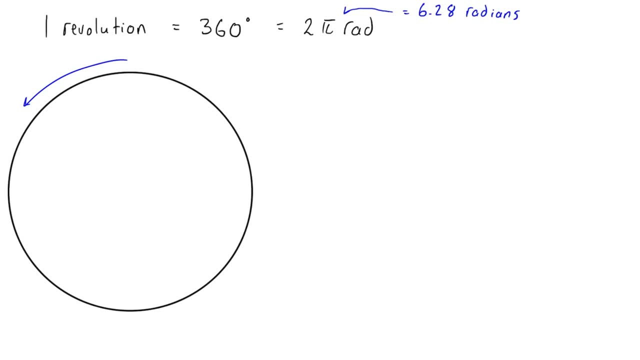 really be leaving in the pi there. It's just a more accurate result. So let's draw on the center of our circle here, and if we wanted to chop this up into degrees, we would literally just hack it into 360 tiny little pieces. Actually, they would be a little bit even. 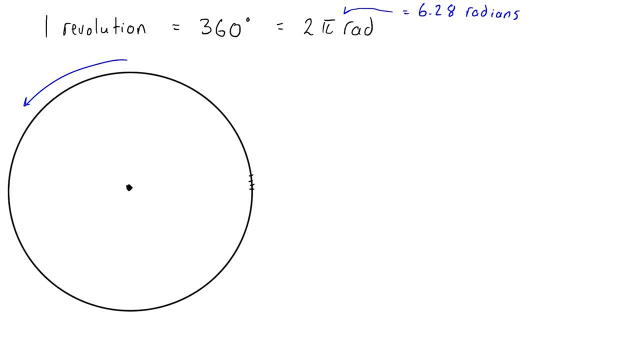 smaller than that. but let's not go the whole way around the circle doing that. But you get the idea. One full pass of the circle is equal to 360 degrees. But let's draw a circle, So let's chop it into 6.28 radians or 2 pi radians, So that would pretty much. 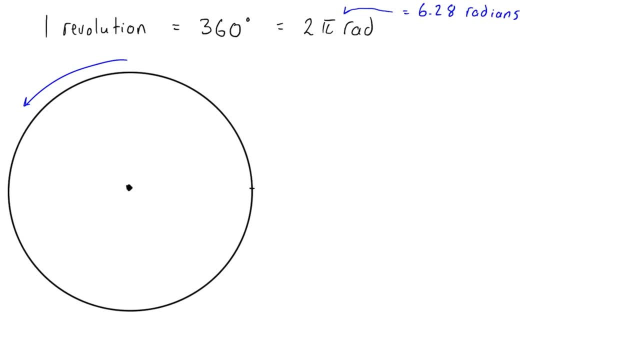 look like if we took the first one here we'd be about like this, then here, then like somewhere over here, somewhere down about there, boom this and then the last little bit like that. So we have the circle chopped into 6.28 parts. but really what we're looking? 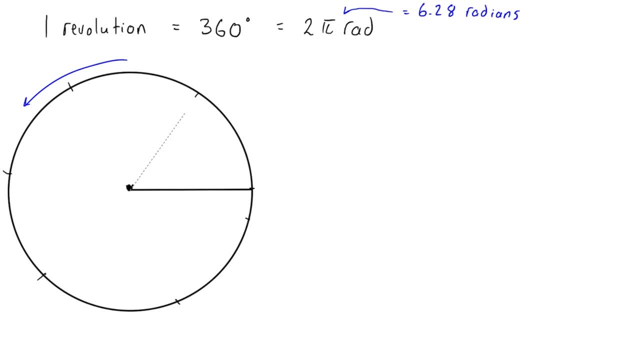 at here is if we draw some radiuses going out from the center of the circle, this is r, and this is r And the radian is pretty cool because for theta here this is equal to 1 radian when the arc is also equal to r. So this curved line here, like this, the 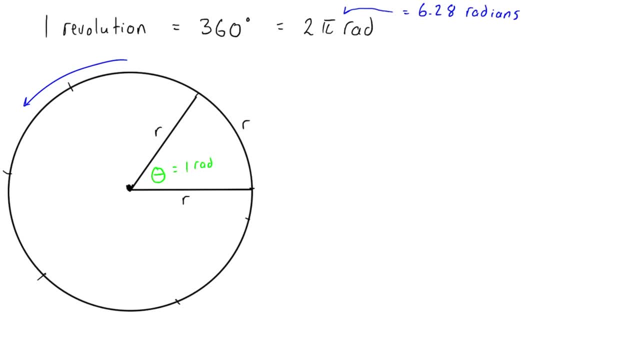 distance from here to here along that circular path is r, then we get 1 radian as the angle that's showing up in here. So that means that this is also 1 radius. this is also 1 radius. this is whoa. 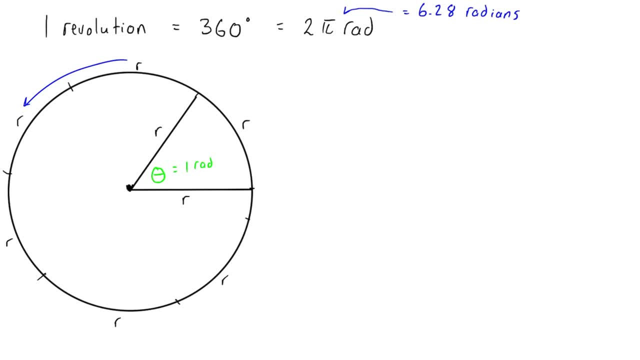 This is also r, this is also r, r, and this little last guy in here is about 0.28 r. right, That would give us 6.28 radians in total to complete the full circle, or 2 pi radians. 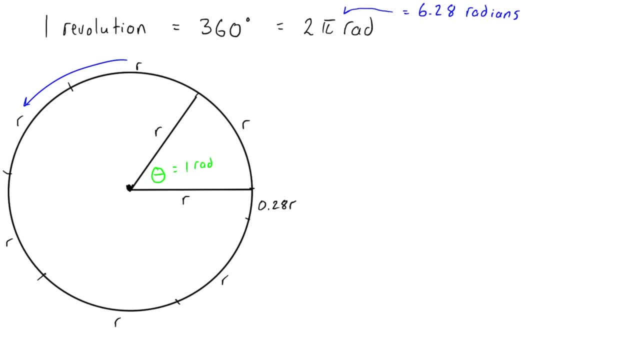 Now, if you want to do some conversions between degrees and radians, the conversion factor is just 360 degrees per 2 pi radians. So if you want to do some conversions between degrees and radians, the conversion factor is just 360 degrees per 2 pi radians. So if you divide 360, divided by 2 pi, you get about. 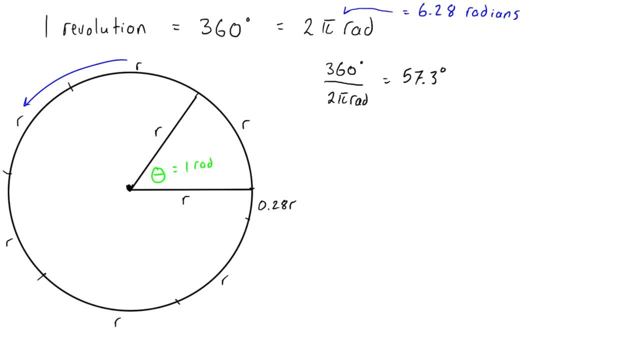 57.3 degrees. So this angle in here is also equal to approximately 57.3 degrees. And if you wanted to convert between revolutions and radians, we just have 1 revolution divided by 2 pi radians. that's equal to each other. This fraction here is unity, so we have radians. 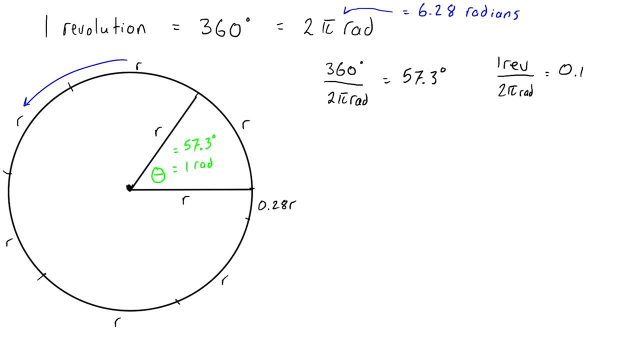 so 1 divided by 2 pi, that gives approximately 0.16 revolutions, which makes this angle in here also 0.16 revolutions. And you can work these all backwards like 0.16 times 2 pi will give you 1 revolution. so vice versa, You can go between degrees, radians and revolutions. 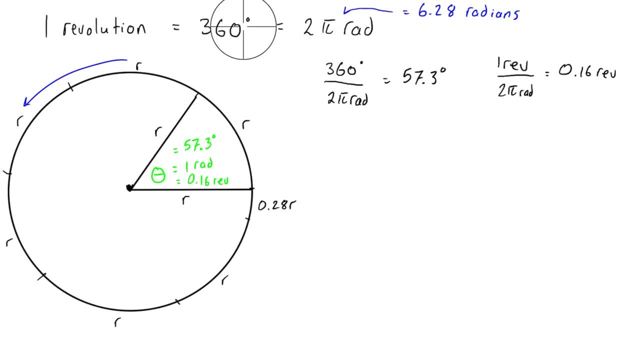 pretty easily just multiplying by unity fractions, using these three values. So let's actually- yeah, let's do some more, Let's do some more conversions along those lines. Let's convert I don't know. let's say, like 4 revolutions. We want to convert this to radians. So what we would do is we: 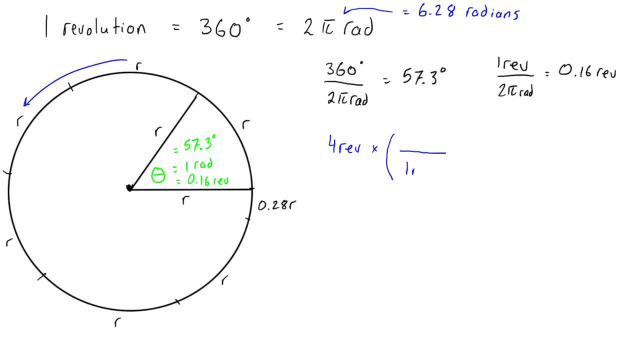 would multiply this by the fraction that has revolutions on the bottom. so 1 revolution times 2 pi radians on top, 4 times 2 pi divided by 1 is equal to 8 pi radians. right, because revolution here cancels out with revolution. 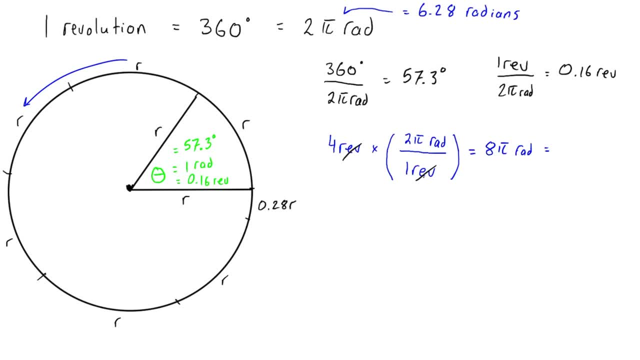 And you can also. you can bring this into. you can get rid of the pi if you want. It would be about 25.1 radians, but anytime you're able to leave the pi in, it's recommended. Now let's do another example. Let's convert maybe 270 degrees and let's put this into. 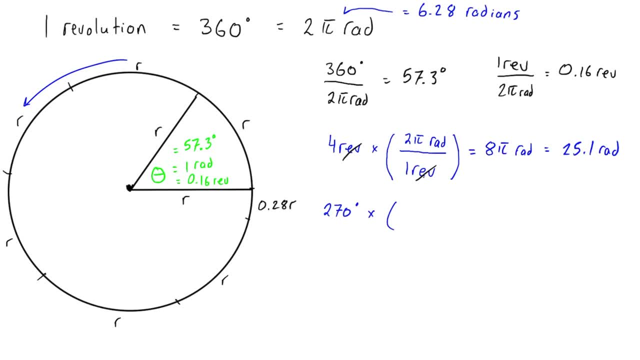 revolutions. So to do that, we would multiply this by the fraction where we have degrees on the bottom, So 360 degrees and revolutions on top. that would be one revolution. so the degrees here are going to cancel out with the degrees there, and 270 times 1 divided by 360 gives us 0.75 revolutions. let's do one more conversion from: 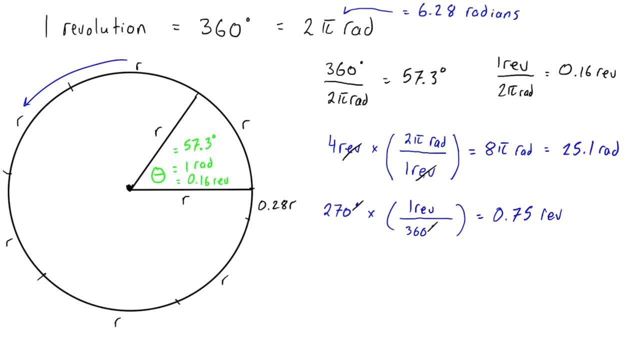 i don't know. let's go from radians to degrees. so let's say we have 8 pi radians- radians, you know, like this number here- and let's convert that to degrees. so we're going to multiply by the fraction where radians is on the bottom: 2 pi radians and 360 degrees on the top. 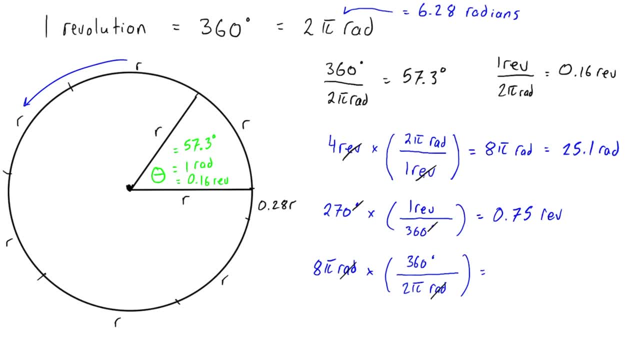 so the radians are going to cancel out when we we can keep this kind of clean like this. pi will cancel out with that pi. so really we have 8 times 360 over 2, so we're going to have 8 times 360 over 2 and we're going to have 8 times 360 over 2. 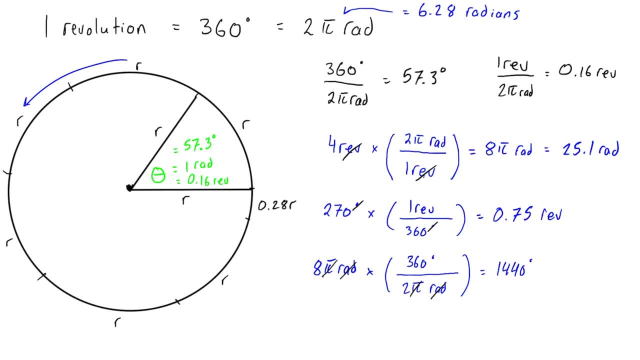 and that's going to give us 1440 degrees, which is the equivalent value, and for those that are familiar with, you know, sports like, i don't know, snowboarding or skiing or something where people are spinning a bunch, 1440 degrees represents four spins, which is exactly what it was up here. 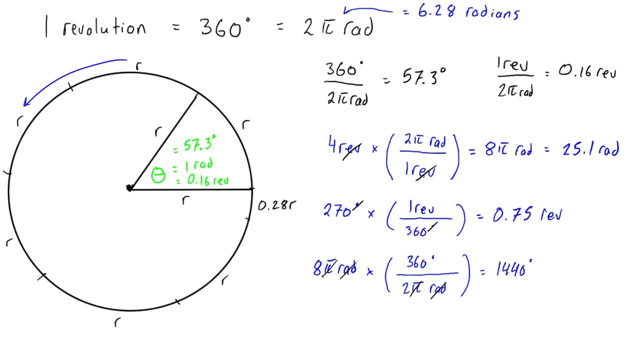 8 pi radians, four revolutions. so there you go, you can just convert pretty quickly between all of those. one other thing that's going to come up a lot in circular motion problems is converting between, uh like introducing a unit of time as well. so, for example, you'll often see: 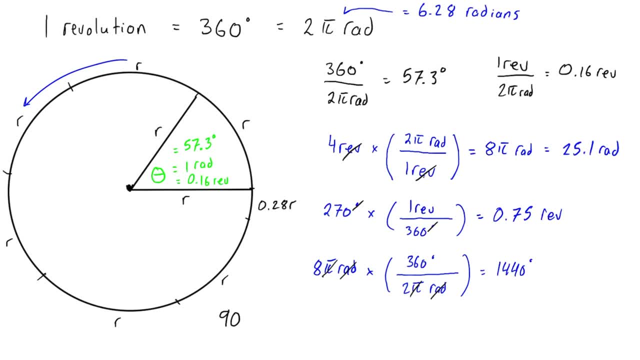 something like: um, i don't know rpm. so let's say we have 90 rpm, this is revolutions per minute. so this would be equal to 90 revolutions per minute, and often we want to convert this into units of radians per second or or something like that, or degrees per hour actually. 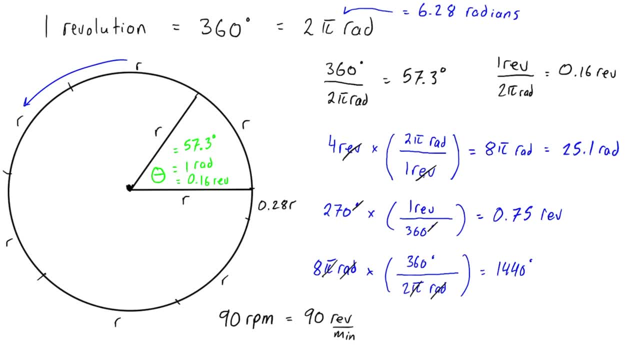 not that, but typically you always want to convert to radians per second uh, and we can do that really easily. so we're going to convert 90 revolutions per minute to uh radians per second. so all we have to do is we have to knock out this revolution term. so again, we put one rev. get it on the bottom.